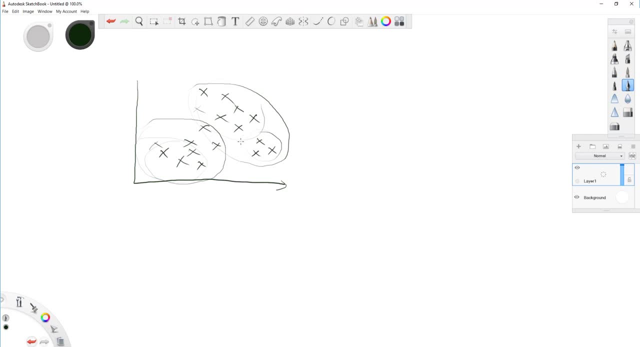 is right here. So you get the point. yeah, So how many clusters do we? do we need to divide this into? Well, you can look at the histogram. actually, if you have the luxury of looking at histogram, or if you have the data you know, just plot, plot it. you know, reshape it into one dimension, plot it. 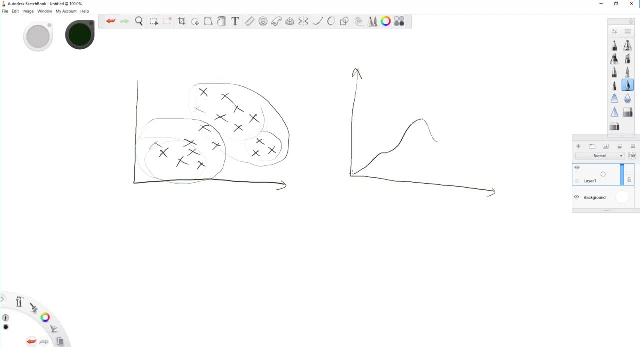 and then if it looks somewhat like this, for example: okay, if your data looks like this, how do you- I mean, It gives you an indication, right? so this is like one, maybe two, three and four, so maybe there's- you need to divide this into four different regions and if you use Gaussian mixture model, you know. 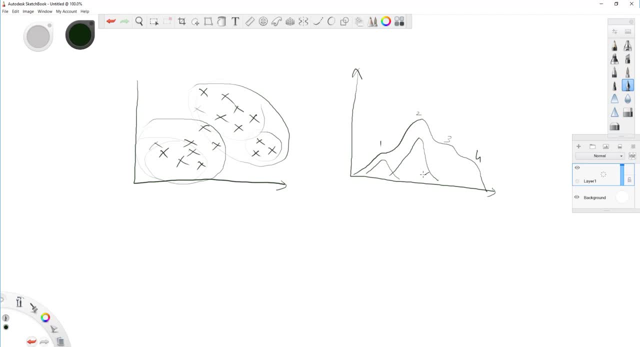 how it's going to fit it right. I mean, it's a bunch of Gaussians and maybe in this case, for Gaussians, you fit this. Now you can fit the same data with even more Gaussians. what if you fit this with multiple? you see a small bump right there up. sorry, let me change the color so it's easier. 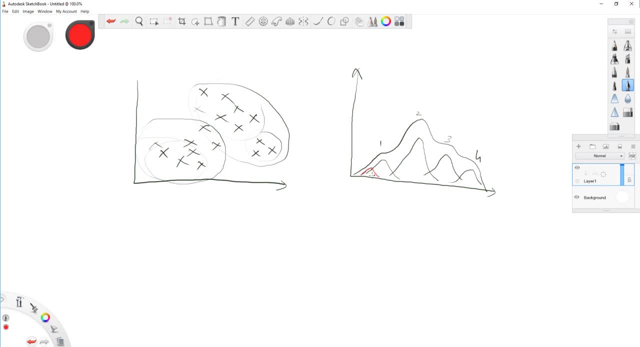 so maybe one peak right here, another right here there seems to flatten a little bit if I read too much into it. I can put one more right here, maybe one right around here, one right here, another one here, another one here and maybe one little one right there. So you can put like one, two, three. 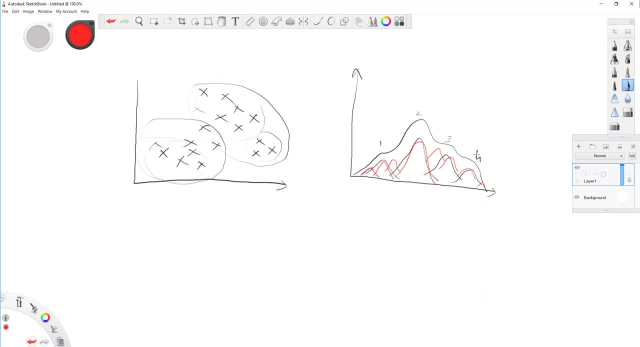 four, five, six, seven, eight and you can really fit like ten of this and this is called overfitting. yeah, So you don't want To. I mean, It may look good actually if you actually use 10 different Gaussians and fit it with your fit. 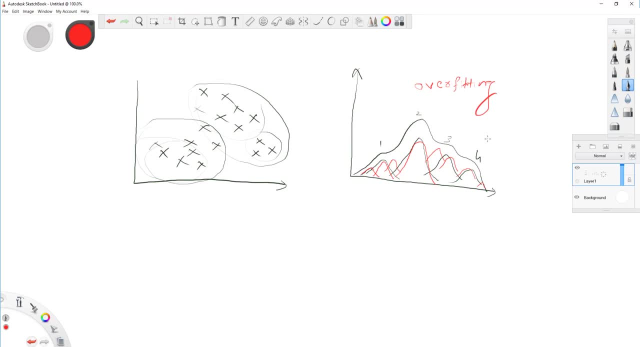 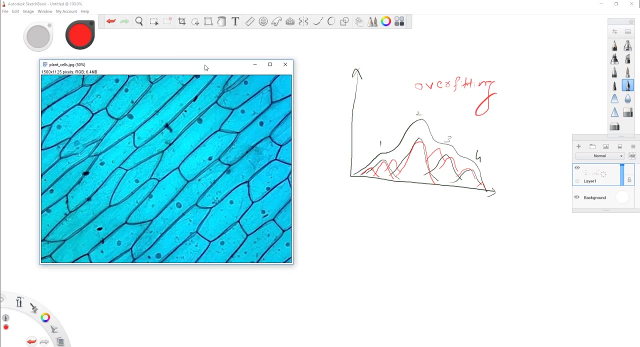 those to your data, to your. it may look like an excellent fit, but this is overfitting what is the true location. so it's very easy: if you're actually working with images, well, let's open an image and see, for example, if you have something like this: well, it looks like there are two regions. 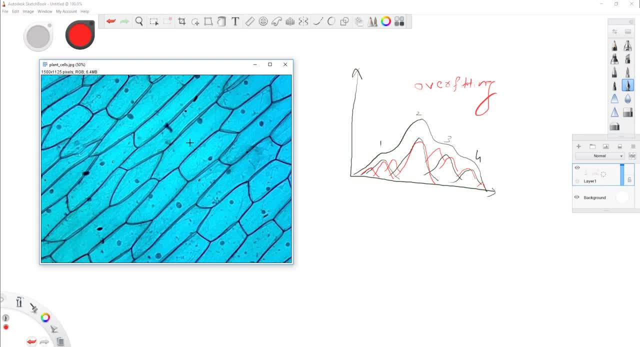 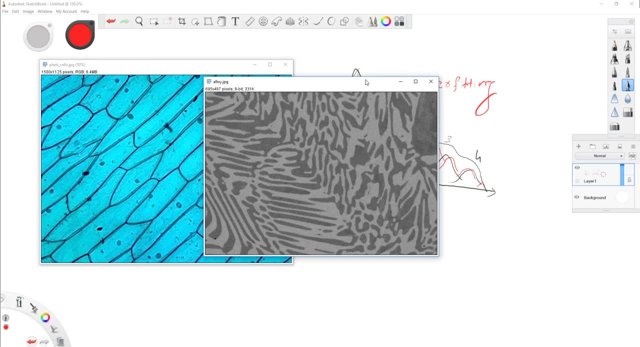 that we can separate right. one is the cell boundaries and the other one is inside the pixels, inside the cell itself. if you have an image like this, this is an alloy and you can see there are two different regions and there is a bunch of noise going along. so in both examples, 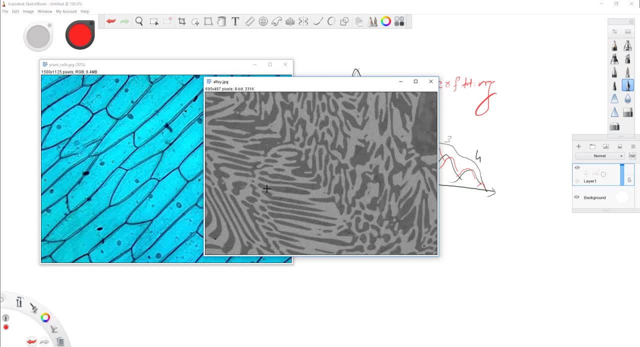 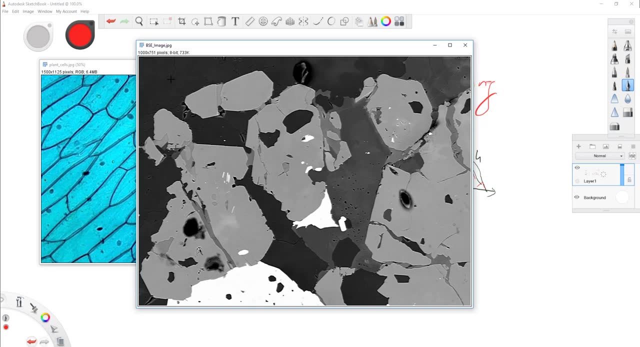 or number of clusters or number of regions is two. now what if you have an image somewhat like this? then visually you can look at this and say, okay, the darkest region is one, although I can say that this region is darker than the darker- you know this one right around here. 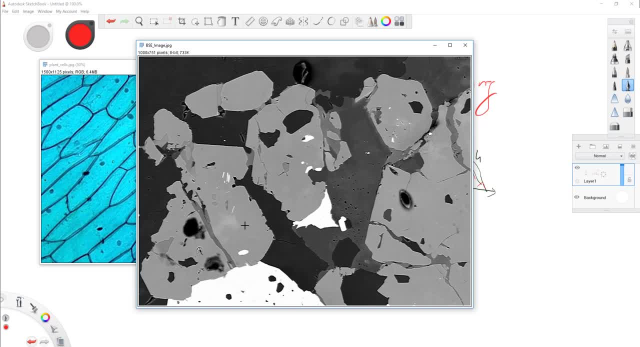 but for now let's say: okay, that's one, this is two and this is three, and four is the brightest and this vein right there can be like five, and I can also see that this region that looks very dark can be six. there can be anywhere from four to six, right, I don't know which one is correct. again, we. 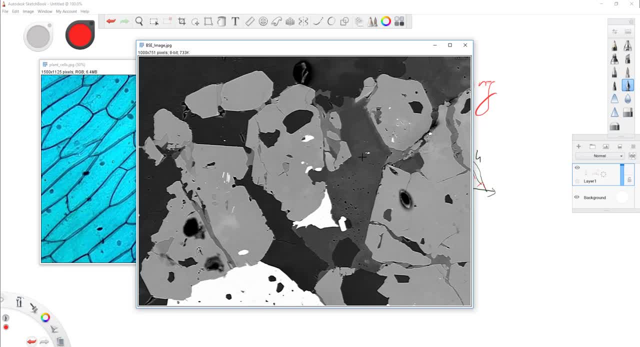 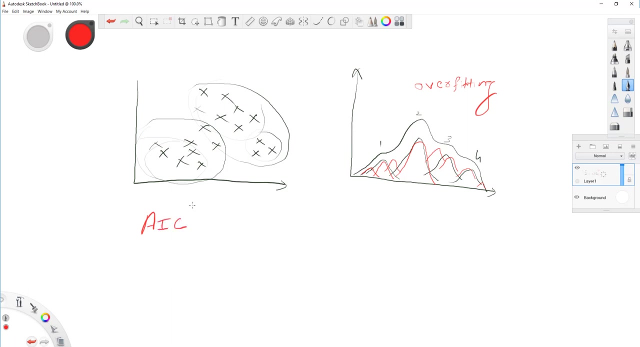 have this issue just by looking at this. not every data is an image, right? I mean in this case, because if I look at theøre замечable, like this year, probability has not been X. but no matter where you look, any distance from thatentes a. 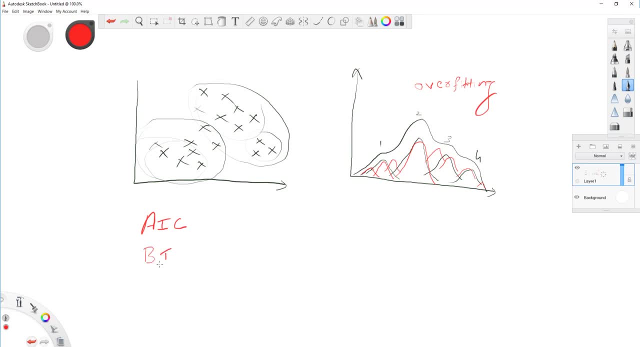 here, but generally this is not a 서정관: say, okay, split this into four or split this into six, so how can we identify, or what guys can we? Bayesian information criteria? okay, and this can be very helpful to pick the right number of parameters, and they both estimate the quality of a model using penalty terms for number of. 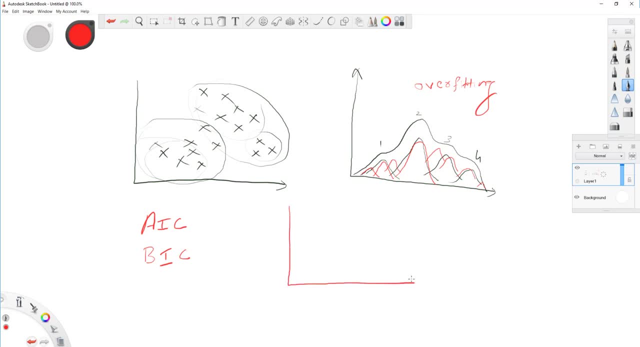 parameters. okay. so all they do is basically they think of: on y-axis you have some penalty term, right, so you have like some sort of a penalty, and on x-axis you have number of parameters, let's say, in our case, number of clusters. it goes from one, two, three and so on, as you increase this, of course, 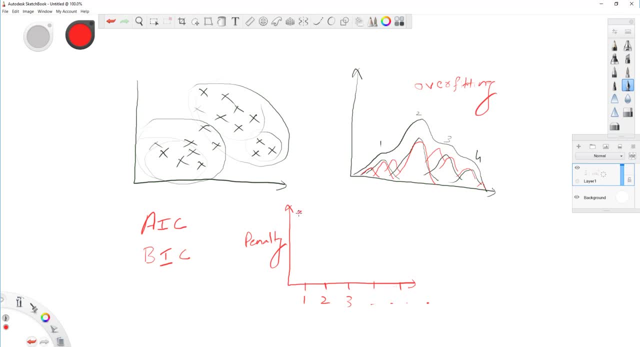 the penalty is very high. if you have very low, and then, meaning it, the fit is not great, okay. and then as you keep adding it, it goes down and down and down and at some point it's like asymptotic. so maybe three is the best number. yeah, I usually pick somewhere around the elbow in real life. 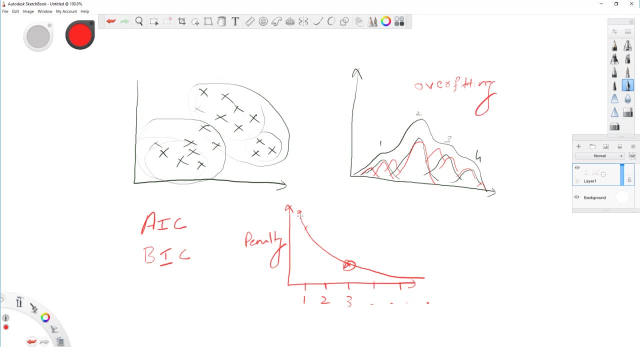 it's not continuous, right. I mean you change it from one, two, three, so this is like one, two, three. well, one two, three, a two, three and so on. So it's not. I'm horrible at drawing, but you get the point. 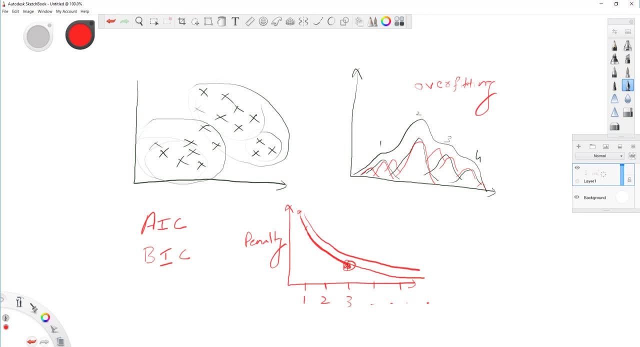 So pick somewhat something right around there. Now, basically, in summary, AIC and BIC: they provide optimal value for number of parameters. if we don't know that, Okay, Now all it's doing is basically, if you think that, okay, this is k, like, number of parameters is k. 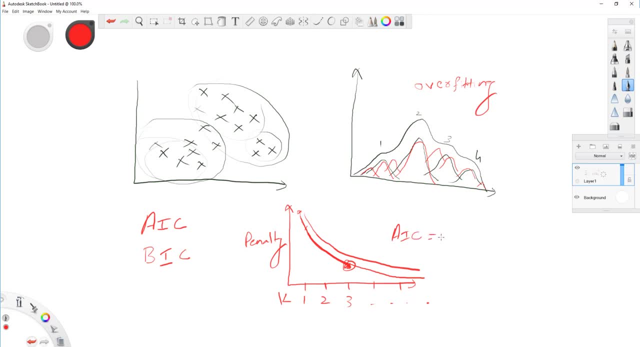 yeah, AIC is nothing but two times k. okay, minus I believe there is a term- two times natural logarithm of the residual sum of squares, or sum of residual squares, if you want to call that okay. So this is: looks at the residuals squares, it sums it and then this is the equation. 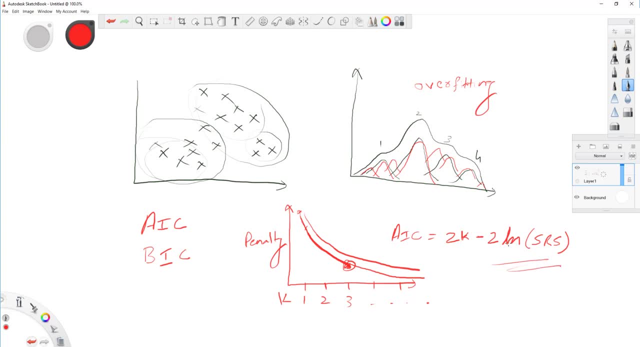 for that. okay, In Python it's just you can just do dot, BIC and then you know. it's pretty easy implementation. But I hope you understand exactly what AIC and BIC mean at a high level and then how we use it in picking the right parameters. Okay, now let's 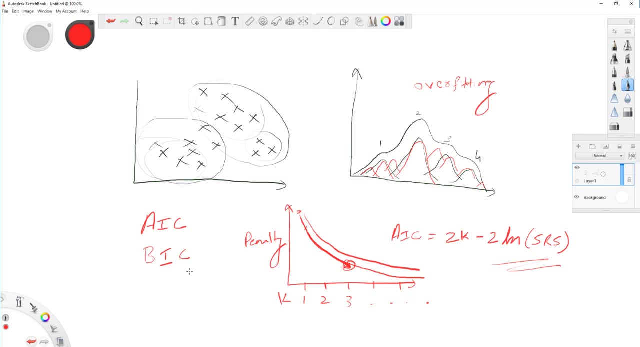 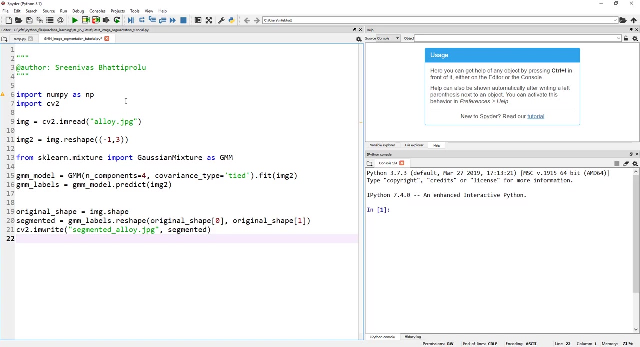 jump into spider and modify our code to use BIC or AIC, And then let's actually plot them. So let me open my spider interface IDE here, And this is the code from last time, actually, Okay, so where we loaded an image, alloy dot, jpeg, and then we reshaped the image. 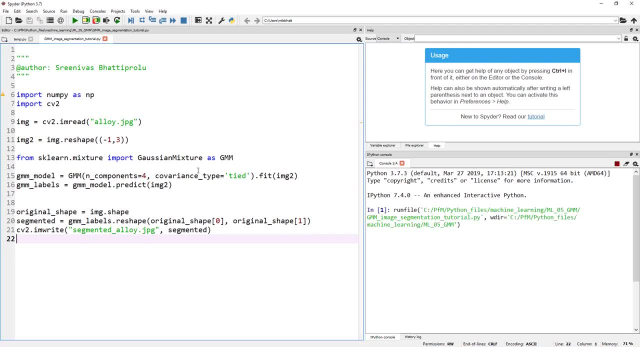 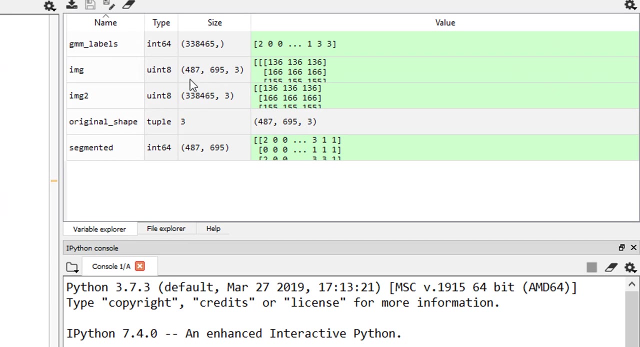 into minus one and three. let me go ahead and run this So you can see exactly what the output looks like. And let's look at variable explorer. So the image is reshaped, And because the original image was 487 by 695, and it's reshaped to 487 times 695, comma three here. okay, 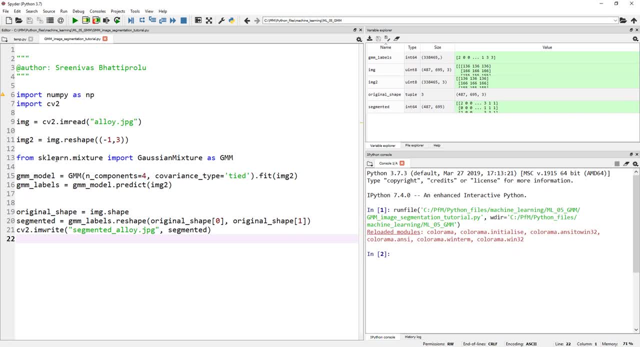 And then we imported Gaussian mixture from scikit learn and defined a model which is nothing but GMM and define the number of components as four. But four is not the right number of components, right? So if I open that image of what do we call it segmented ally, let me go ahead and import that. 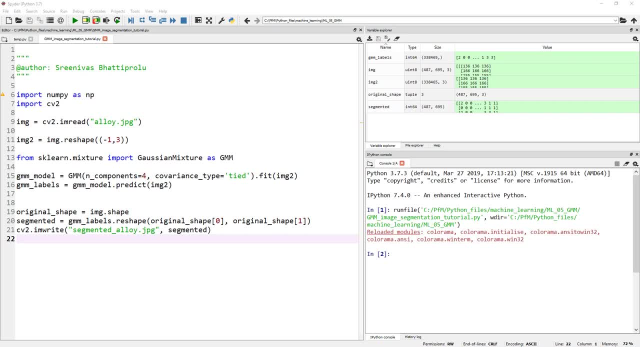 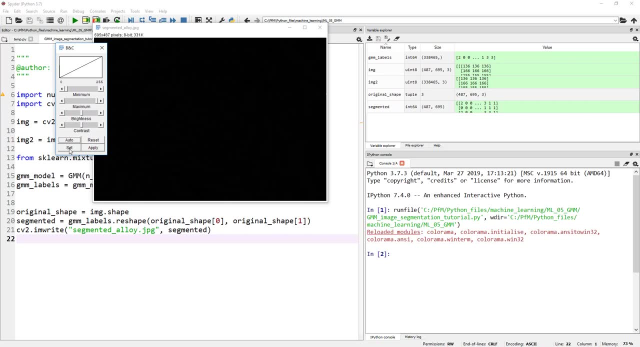 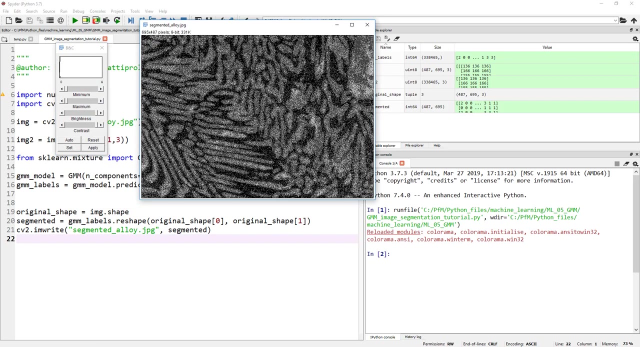 image And you can see how it looks like this is supposed to be a binary image. Let me change the brightness and contrast to zero to four, because we have- and you see that's not a great segmentation. Yeah, because we are segmenting it into multiple regions. it should be only two. So now, if I actually go and change the 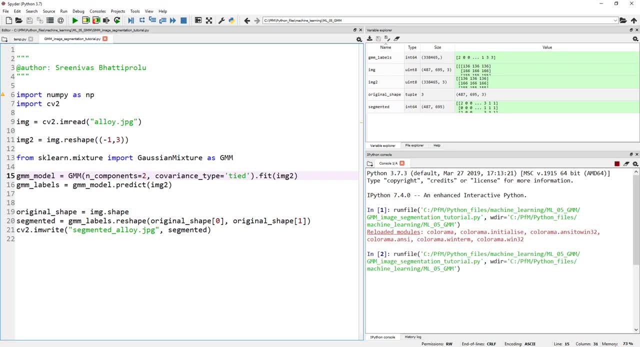 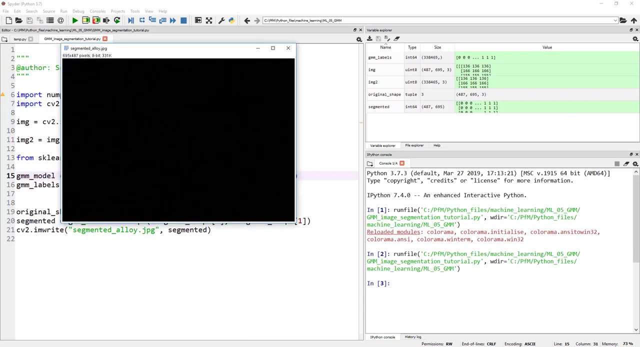 number of components to two and run this one more time and let's kill this image so I can open the next one. Okay, so now let's open this image again, the new image that got generated, segmented alloy. Let me go up and open it And there you go. Let me adjust the brightness and contrast: set zero to. 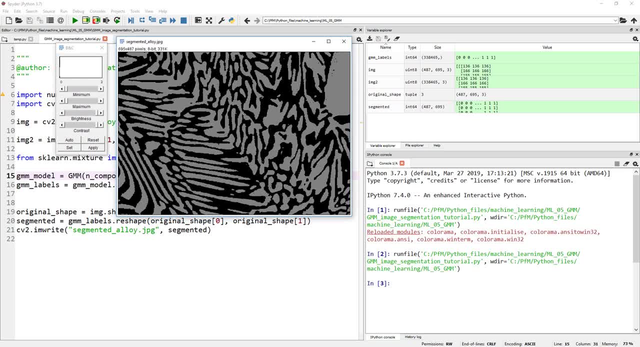 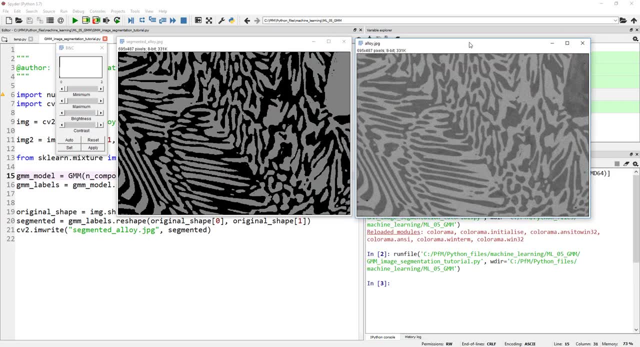 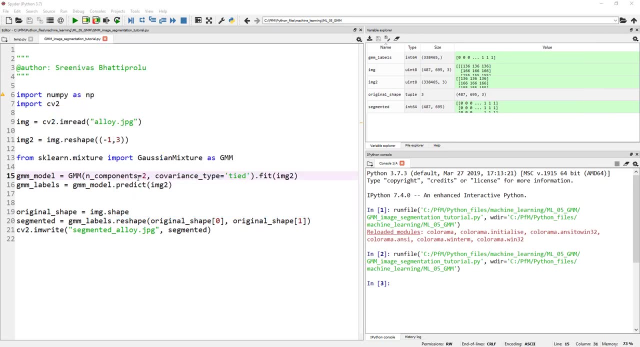 two. Okay- And this is an amazing segmentation- Okay, And you see the original images right here. So this is the original image And this is the segmented image. It's a pretty good segmentation. So how do we know that? again, we have two components. two components is the right one. So 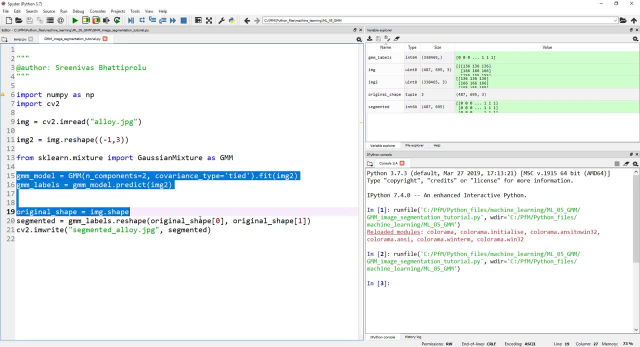 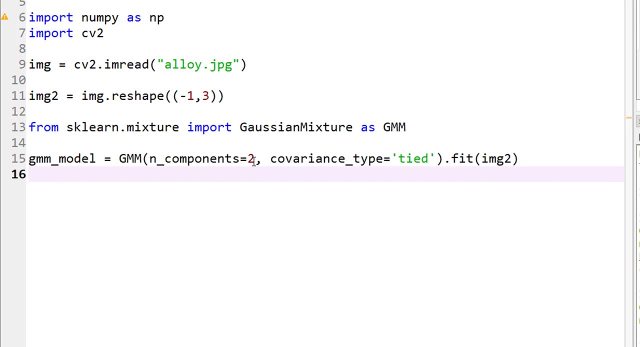 instead of doing all of this, let me remove that. And well, actually, let's remove this label spot. And now let's modify the code to actually change the number of components from one all the way through 10.. Okay, let's go from one component to 10 components and see how that BIC or AIC looks like. So for 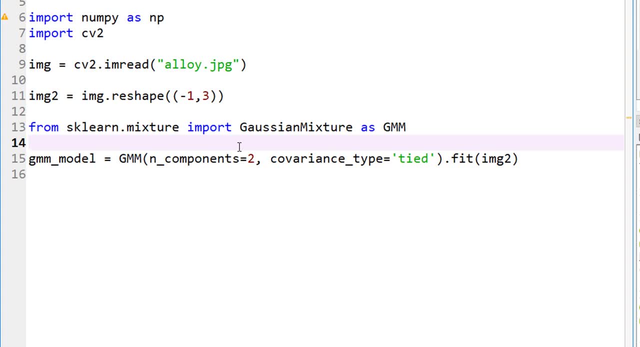 that let's go ahead and define number of components Instead of defining it inside here. I'm going to just define a range. Okay, the range is going from one through 10, let's say okay, so it changes 10 times in here. So now that I've defined this, let's iterate it. 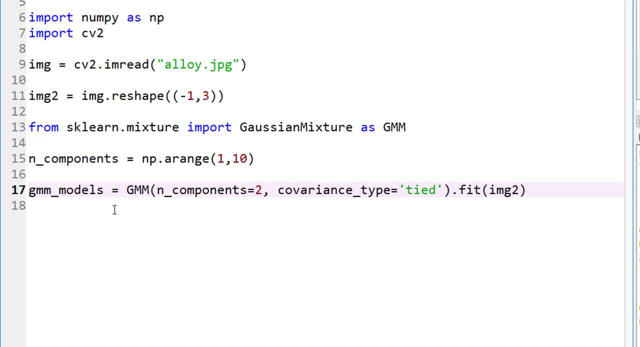 inside this GMM model. Okay, let's change this to models, because we have more than one And let's iterate this in here. So let me put my square brackets up there, And GMM means the total number of components. So this is the model we're going to use. 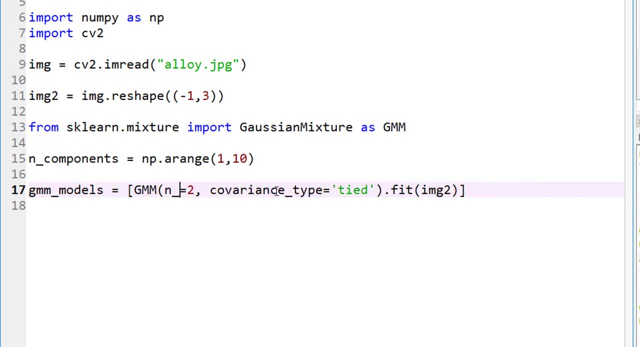 and instead of number of components it's got to be n. Okay, and let's cycle through and in a second, okay, and and my covariance, I'm going to leave it to tide fit. image two: that's good, Everything looks good there. for n in and underscore components: Okay. so all it's doing is changing n. 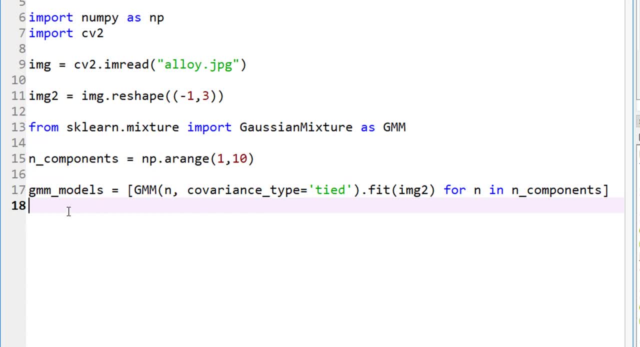 from one through 10. And then running this. that's pretty much it. So once it's done, let's go ahead and plot it. So from Matt, did we do that here? No, let's from matplotlib Import pi plot as PLT. 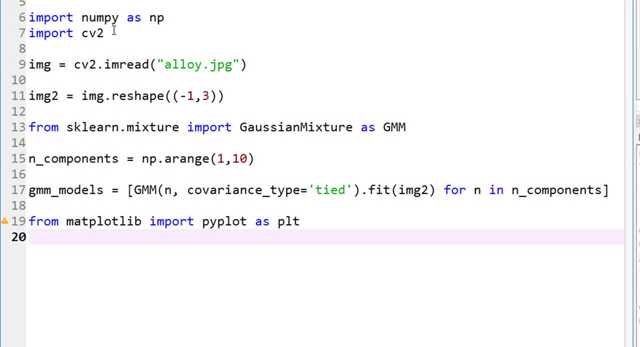 Okay, Normally I define this, import, this library right. You know, on the top It's one of the key libraries: PLT, dot plot. And what are we plotting? number of components on x axis. let's do number of components And let's plot. 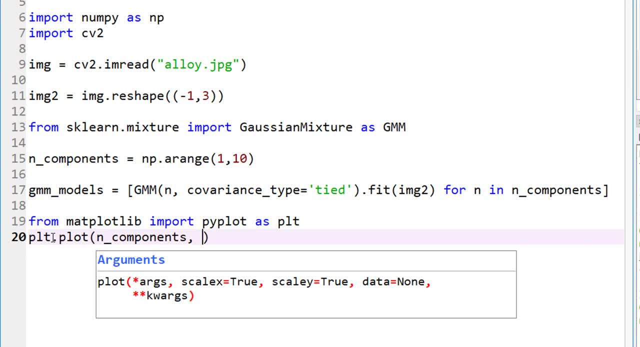 plot that against BIC, But then we need to iterate through different BIC. So the way we can, the easiest way we can do, is: let's define m And BIC of image two right, our input data is image two, that's our raw data. calculate the BIC image two for m in GMM. what did we call it? models? 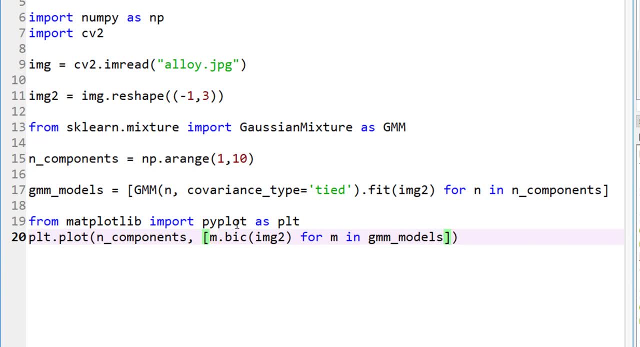 I think that should do right and be. I see, okay, And let's label this, We don't need to. I mean, let's label this as BIC, So we know exactly what we are plotting. I think that looks good, Let's go ahead. 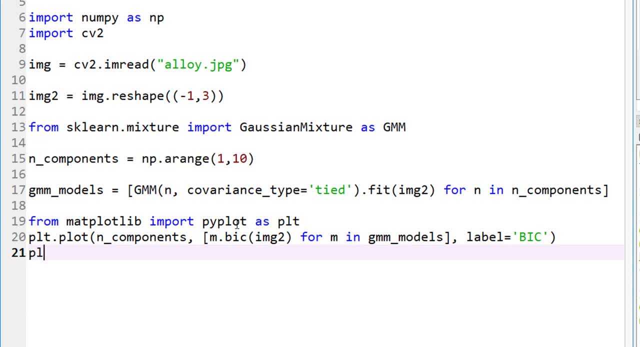 and plot it. And if you want, you can label the x axis. okay, to make it X label. And let's call this n underscore components. That should do. I'm not plotting a. I see to plot a. I see it's. 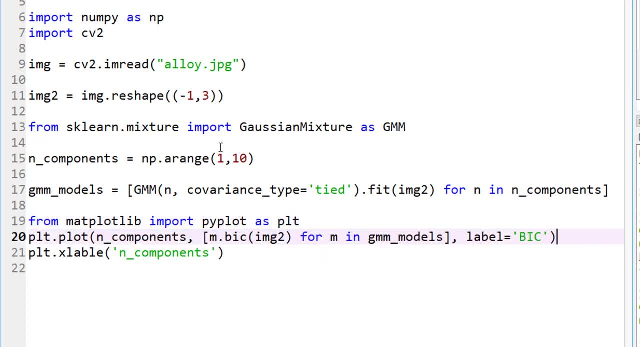 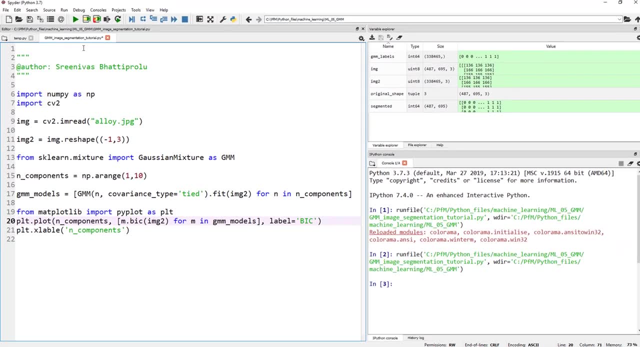 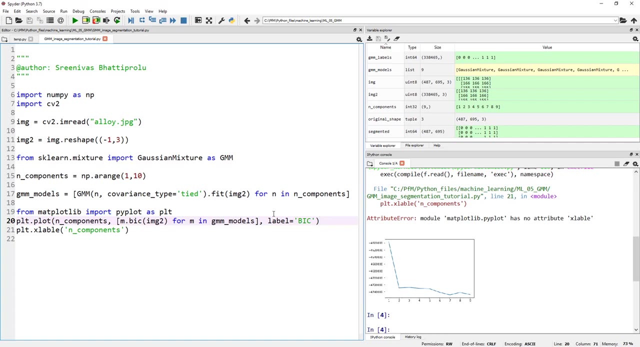 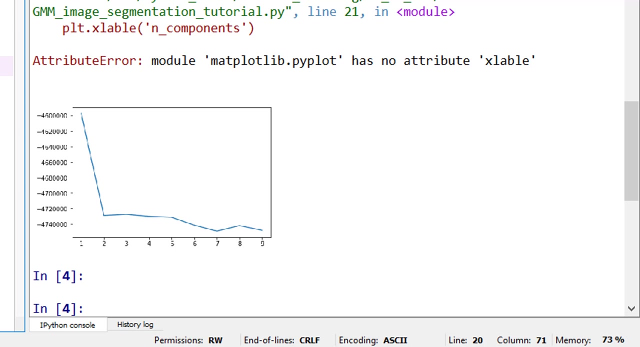 again, you copy this line and change this BIC to AIC. That's pretty much it, So let's go ahead and run this. It may take a little while because it's going to iterate through 10 times, So let's run it, Okay. so obviously I seem to have mistyped here, you know, instead of L-A-B-E-L,